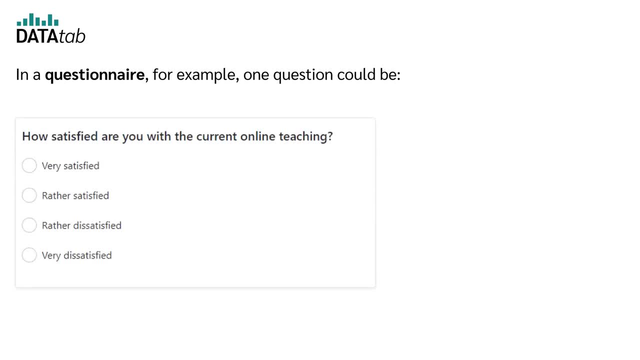 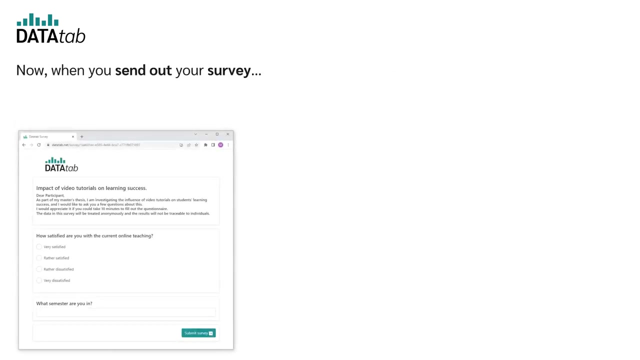 for example, one question could be: how satisfied are you with the current online teaching? Very satisfied, rather satisfied, rather dissatisfied or very dissatisfied? So you would define the possible answer options Now, when you send out your survey and get the results. 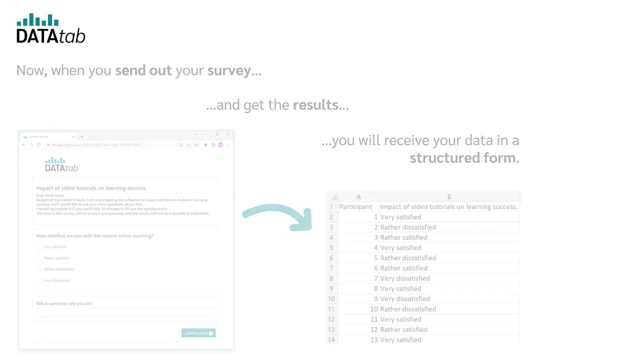 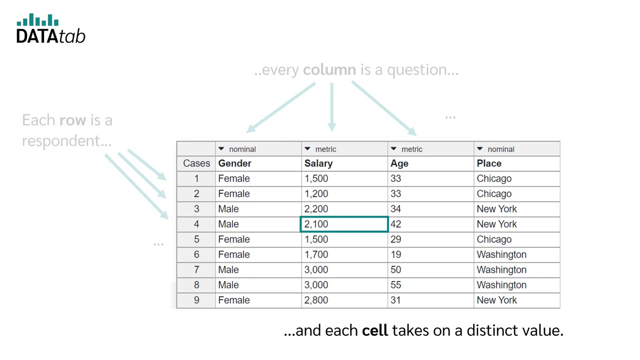 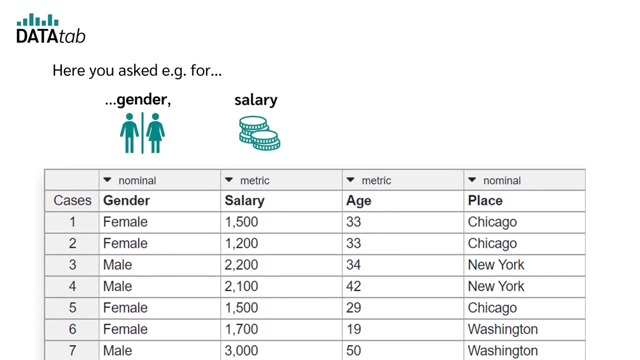 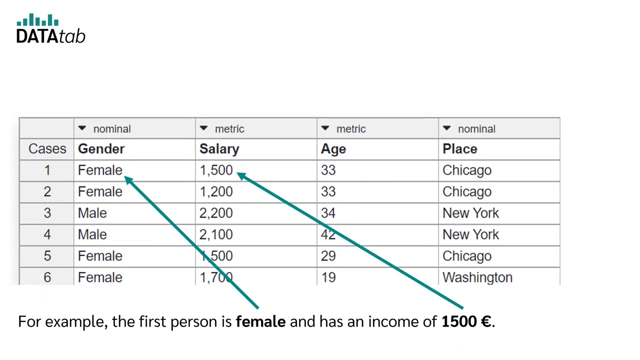 you will receive your data in a structured form. Each row is a respondent, every column is a question and each cell takes on a distinct value. Here you asked, for example, for gender, salary and age of your respondents. For example, the first person is female and has an income of. 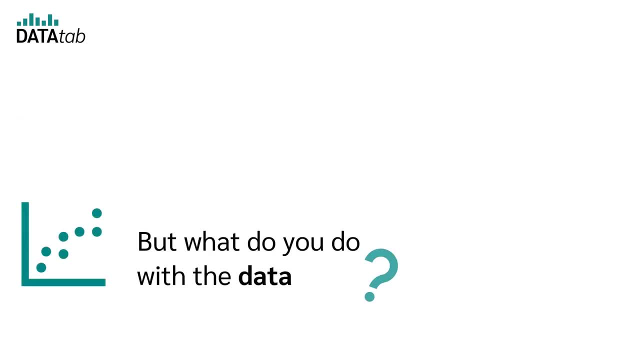 1,500 euros. But what do you do with the data? Depending on the insights you want to gain, you can either work in a descriptive, hypothesis testing or exploratory way. Let's start with the descriptive statistics Based on your population. 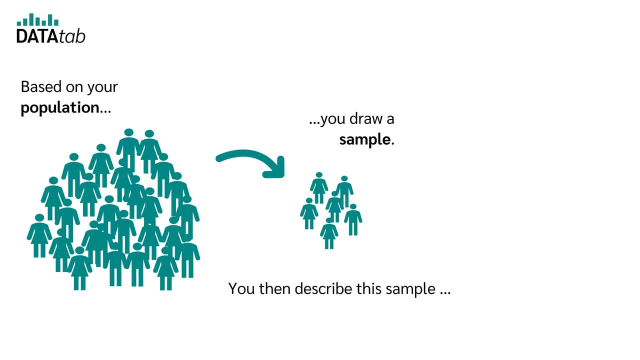 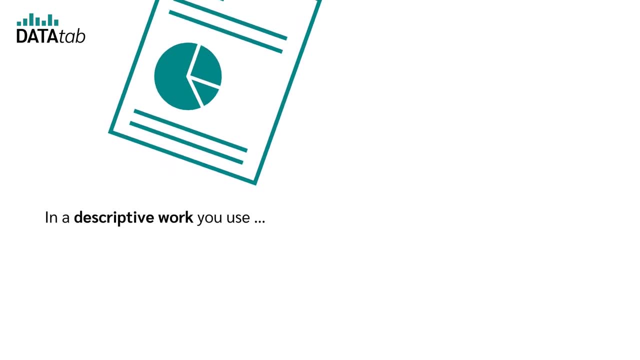 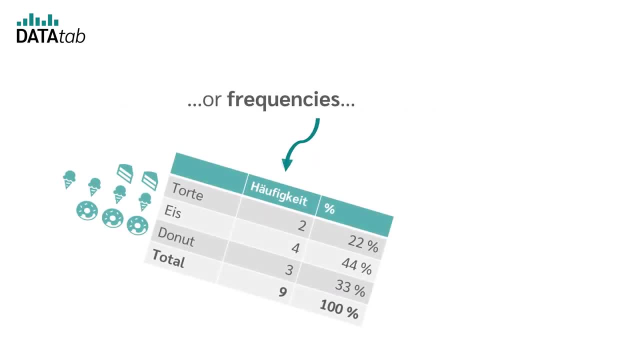 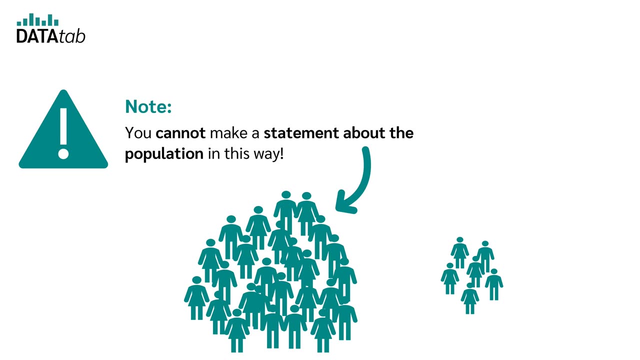 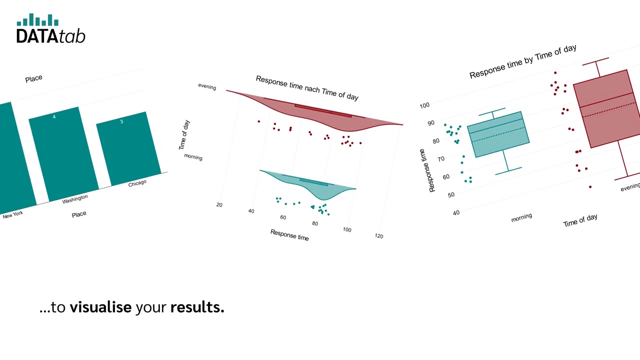 the mean value, the standard deviation or frequencies to describe your sample. Note. you cannot make a statement about the population in this way. Of course, in Descriptive statistics you use diagrams to visualize your results. What does this look like in a hypothesis testing study? 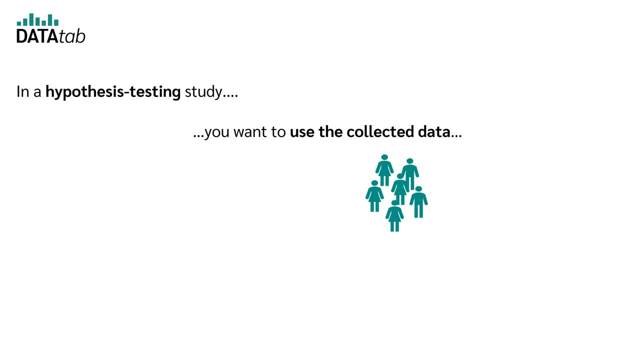 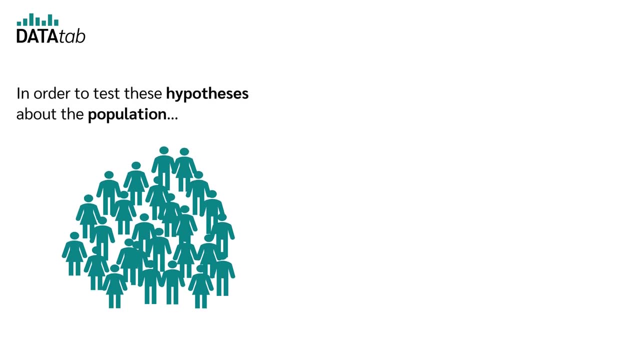 In a hypothesis testing study, you want to use the collected data to test hypotheses about the population. In order to test these hypotheses about the population on the basis of a sample, you use a hypothesis test. This could be, for example, a t-test, an analysis of variance. 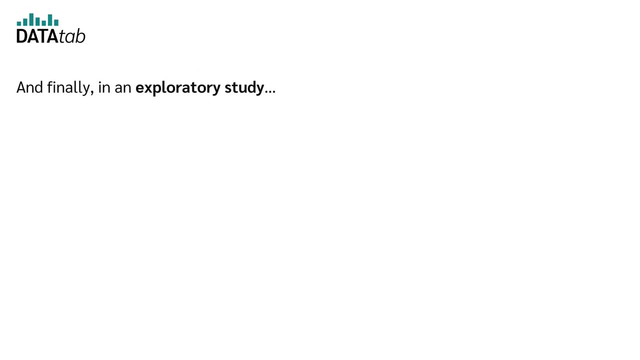 or a correlation analysis. And finally, in an exploratory study, you want to identify unknown patterns from the data collected. For this you use, for example, a cluster analysis. Of course, you can also combine the three areas of descriptive hypothesis, testing and exploratory. 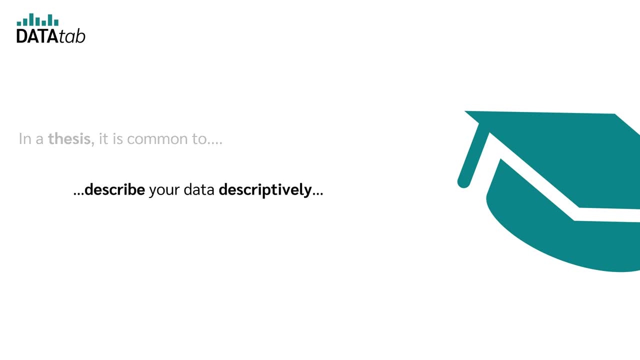 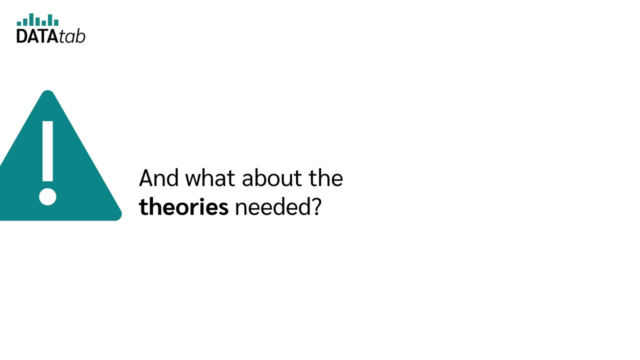 In a thesis, it is common to describe your data descriptively and then test your hypotheses using hypothesis tests. But now we have omitted a very important part: What about the hypothesis, What about the literature, research And what about the theories needed? 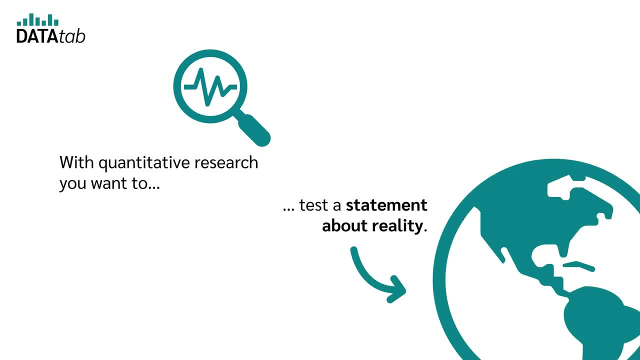 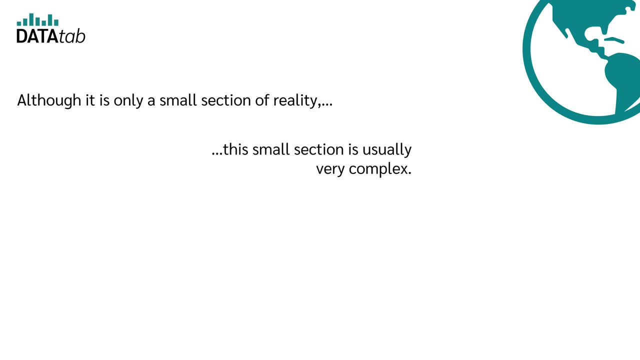 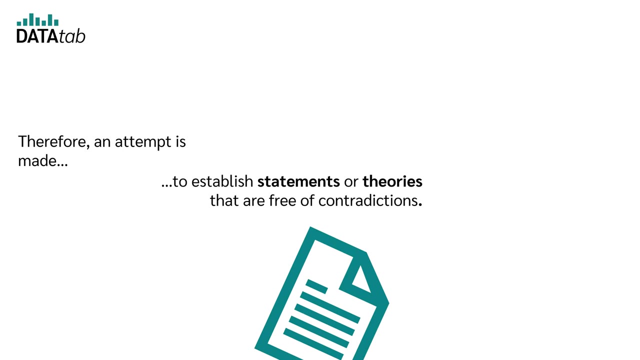 With quantitative research you want to test a statement about reality, Although it is only a small section of reality. this small section is usually very complex. Therefore, an attempt is made to establish statements or theories that are free of contradictions. So reality is very 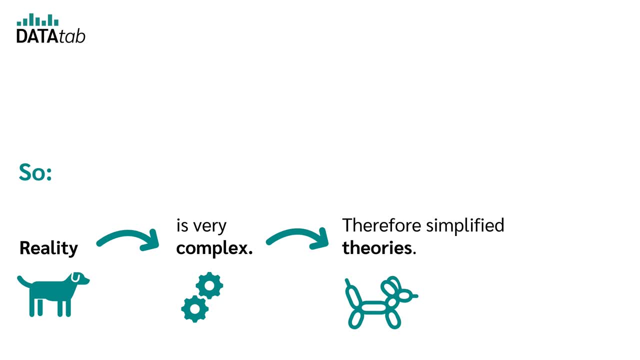 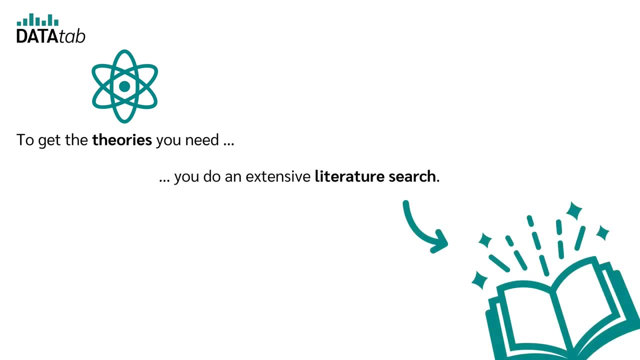 complex. And what about the theories needed? With quantitative research, you want to test a statement. complex, Therefore simplified theories. But how do I get the theories? I need To get the theories you need. you do an extensive literature search. You can then derive your 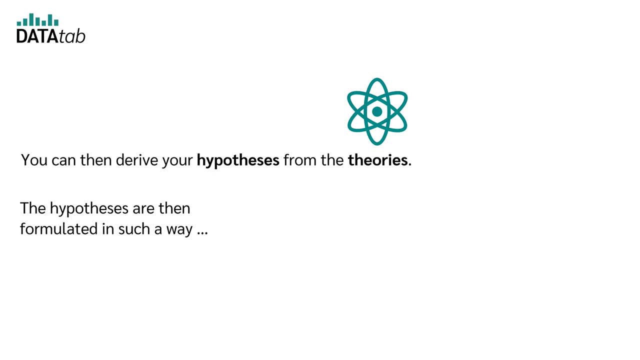 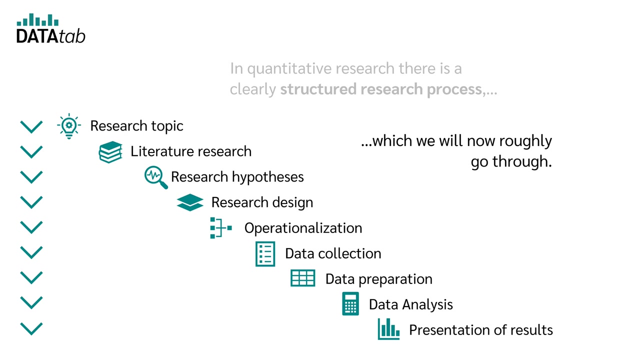 hypotheses from the theories. The hypotheses are then formulated in such a way that they can be tested using collected data. Of course, you have to do the literature review at the very beginning of your research. In a quantitative research, there is a clearly structured research process, which we will now. 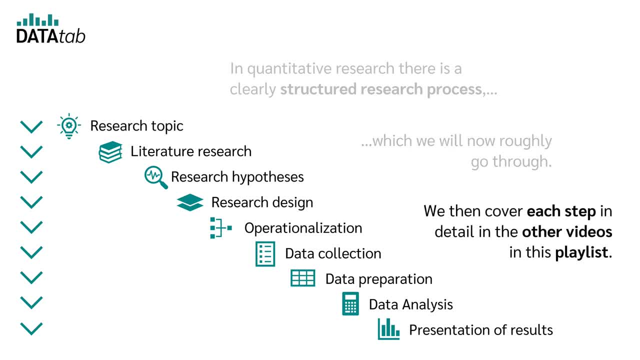 roughly go through. We then cover each step in detail in the other videos in this playlist. At the very beginning you have to find a research topic. Then comes the literature research. In practice, these two steps are often carried out in parallel and not one after the other. 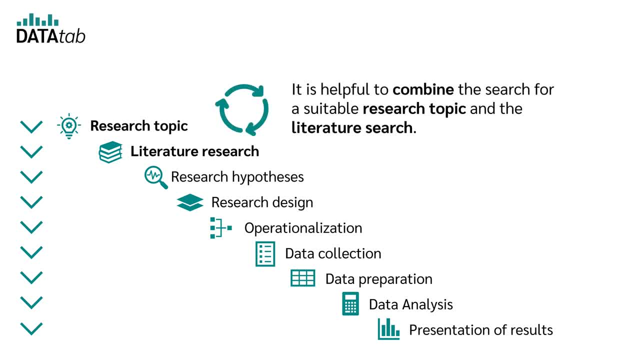 It is helpful to combine the search for a suitable research topic and the literature search. From the literature research you can work out the state of research and the theoretical background and derive your hypotheses. Then you come to your research design. Here you define how you want to.